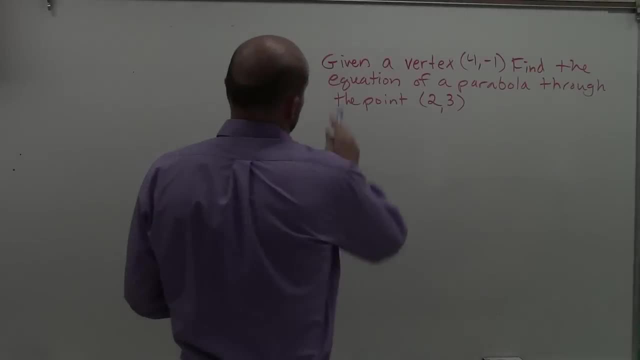 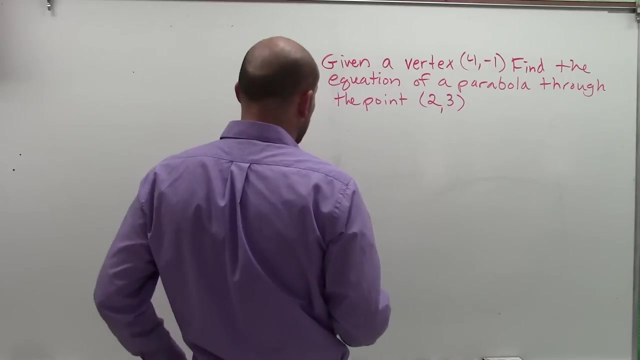 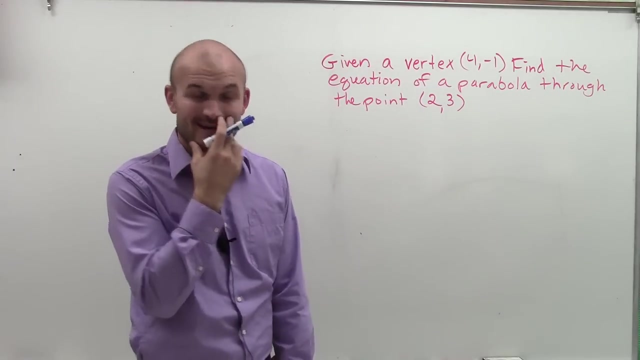 Given a vertex 4, negative 1, and find the equation of the parabola through the point 2, 3.. Huh huh, Good one. right Before I get into this, I want to kind of do a quick little review of linear equations. 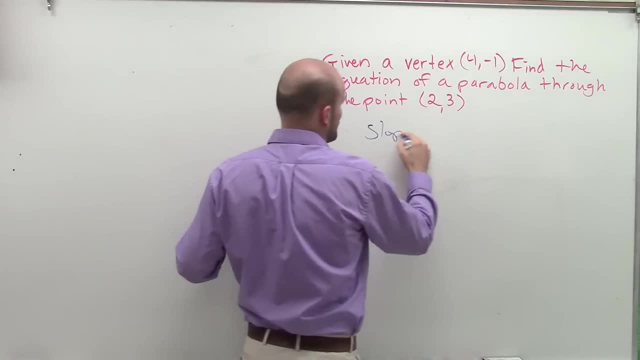 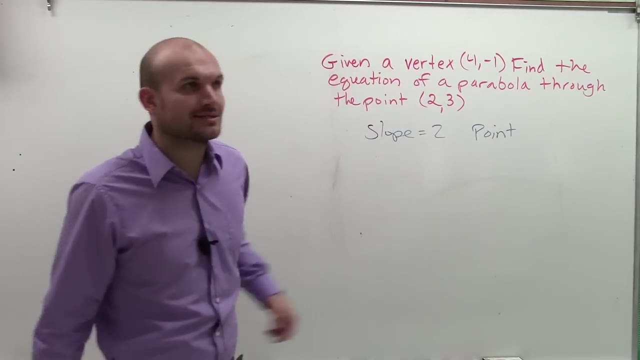 What do we do when we have a linear equation? Let's say I give you the slope equal to 2.. And I'm totally making this up, so I don't even know if it's going to work. And let's pick a point: negative 1, 3.. 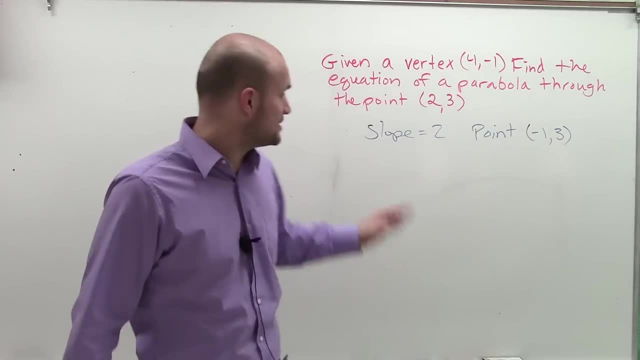 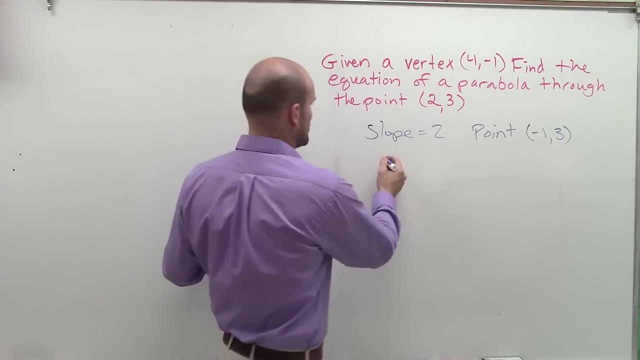 Remember, if I say, find the equation, find the linear equation of a line that has a slope, 2 and a point, what we'd like to do is we can use the point-slope method. Well, the point-slope equation is: y minus y1 equals m times x minus x1.. 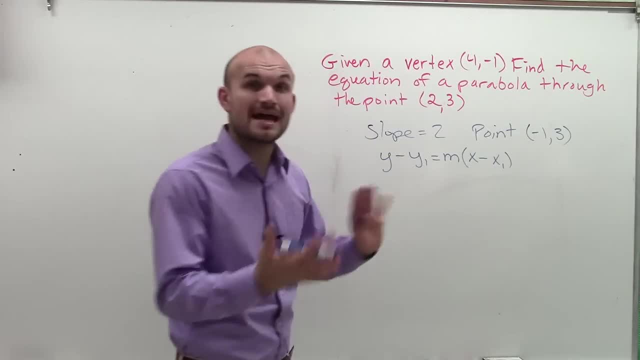 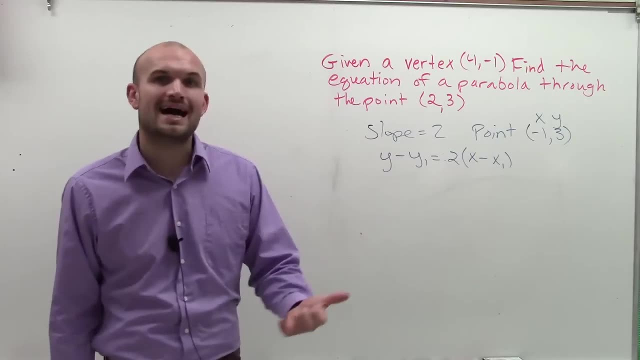 And what we do is we're going to find the slope, And what we do is we plug in 2 for our slope right, because m represents slope, And then we plug negative 1, 3 because, remember, a point on a line is made up of infinite many points. 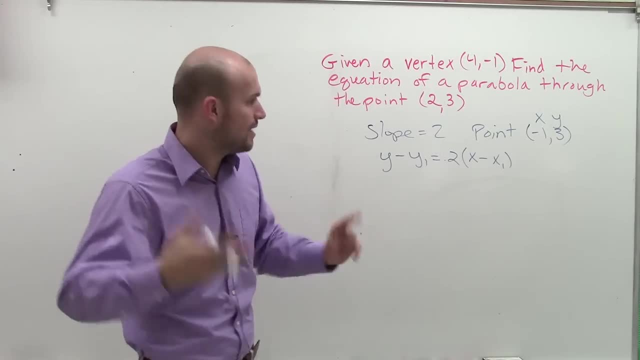 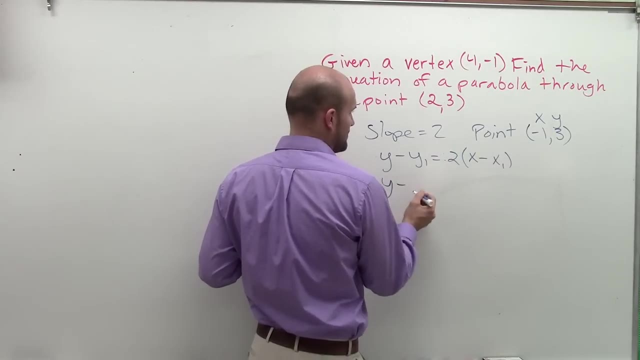 So if I'm given a point, I can plug that in for x and y And in point-slope form I'm going to plug my x and y in for x1 and y1.. So what I do is I write y minus I guess, leave that down there: y minus y3,. 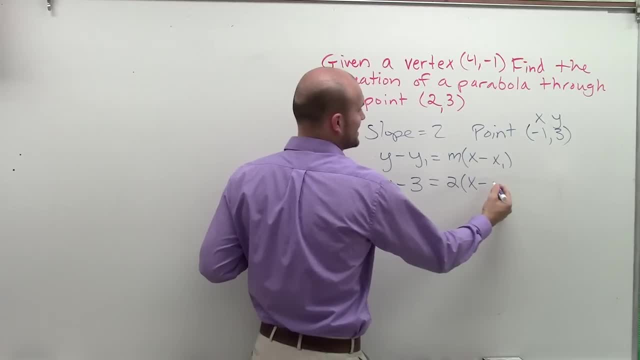 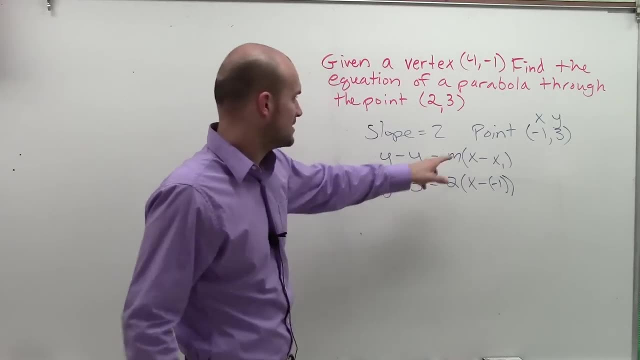 equals 2 times x minus a negative 1.. Then what we do is we simplify right, So we do a distributive property, So that's 2 times x, which is 2x, And then we have that's going to be a positive 1.. 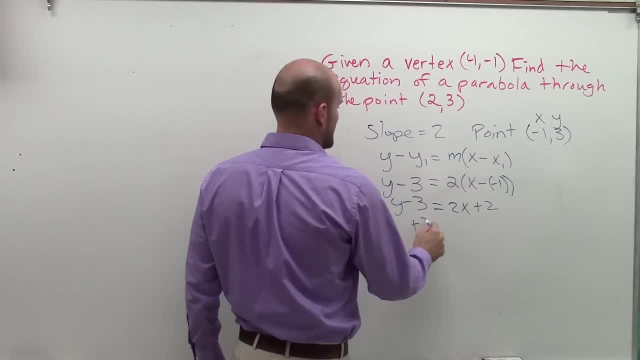 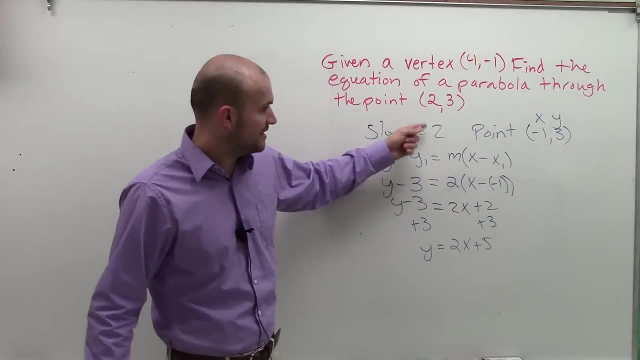 2 times positive. 1 is 2.. y minus 3, add 3, add 3.. My equation is 2x plus 5, right, So we take our given, we plug it into the equation. We also take our other given. 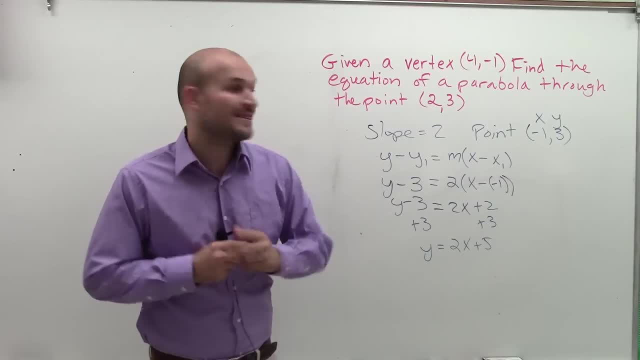 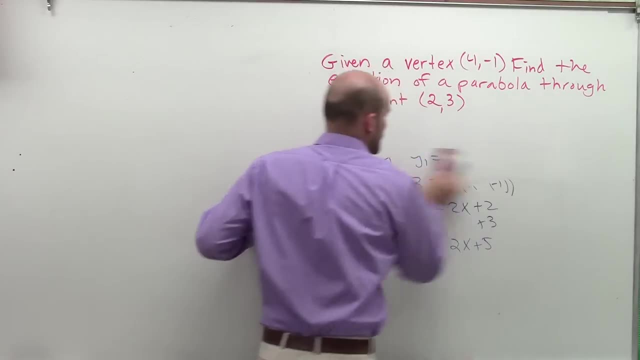 And which is a point, and we plug it in for x and y. Well, guess what? This problem is almost identical. Well, not identical, but it's parallel to the same type of process. So what we're given is: we're given a vertex and we're given a point. 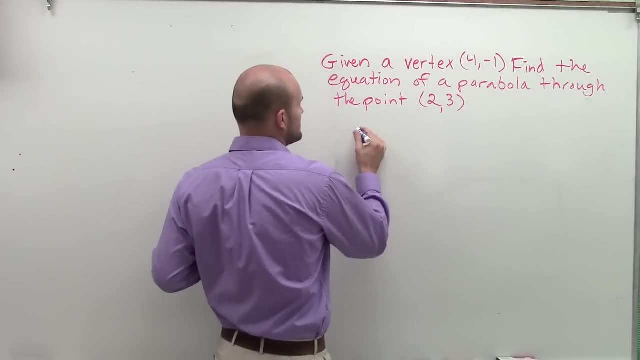 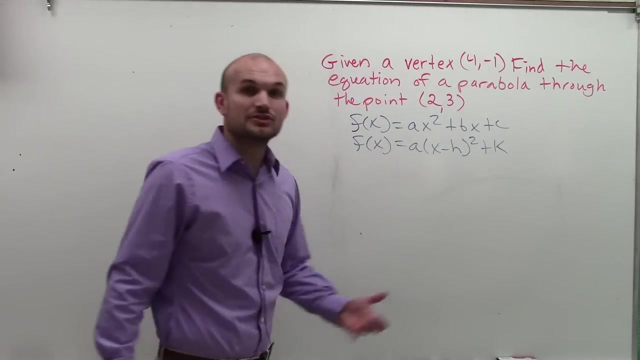 Now we need to determine what are we going to plug that into. So we've talked about two different ways to define a quadratic. Here is our definition of a quadratic and here is our standard form. And I think whenever we started introducing standard form, 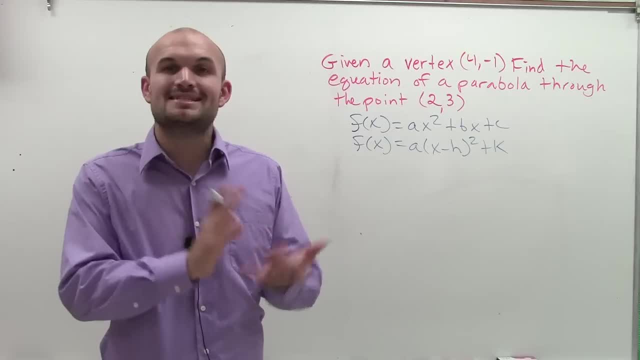 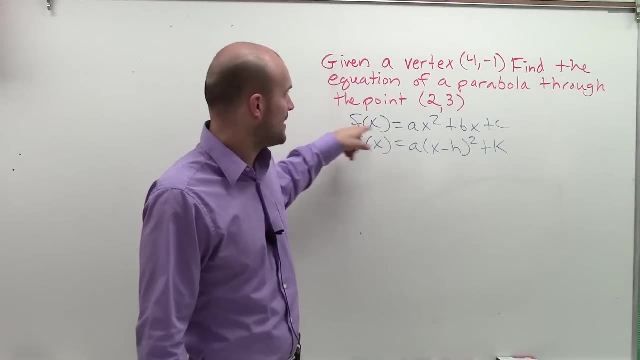 we always praised standard form because it's so easy to find the vertex. The vertex is h, k, right, So what do you think is going to be the easiest form to use for this If I want to find out the equation on my parabola? 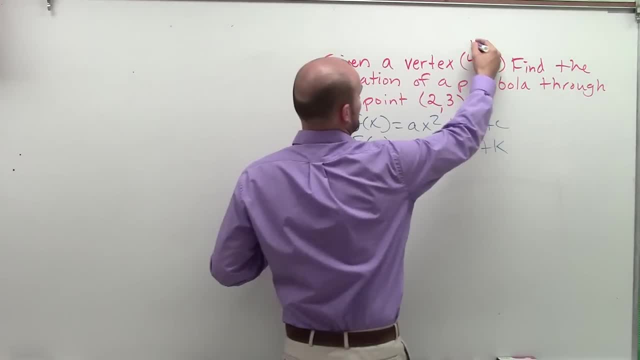 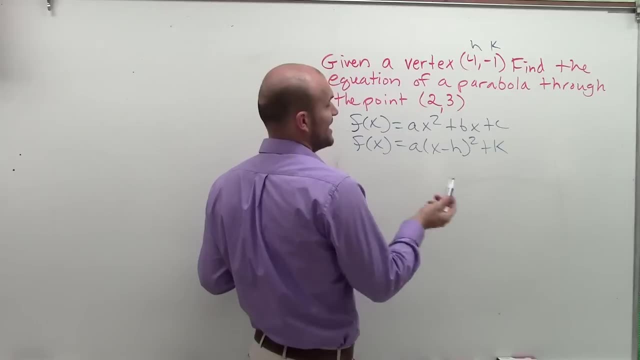 I'm going to want to plug in my vertex for h k, h k, right there. So that's exactly what I'm going to do. I'm going to plug in a negative 1 for k and a 4 in for h. 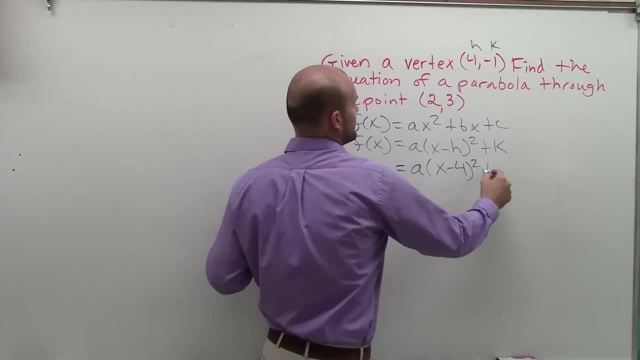 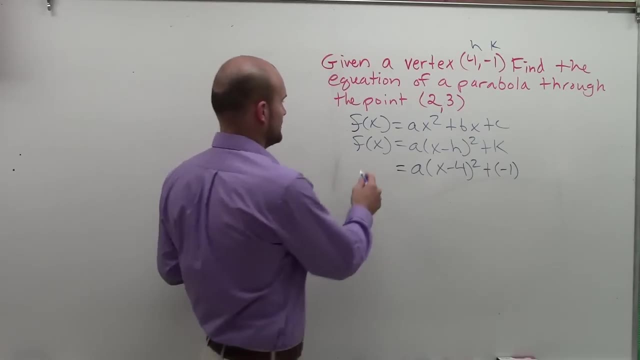 So I have a times, I have a times x minus 4, squared plus a negative 1, and that equals f of x. Now the next important thing is: all right, so that tells us there. That doesn't give us the full equation, though. 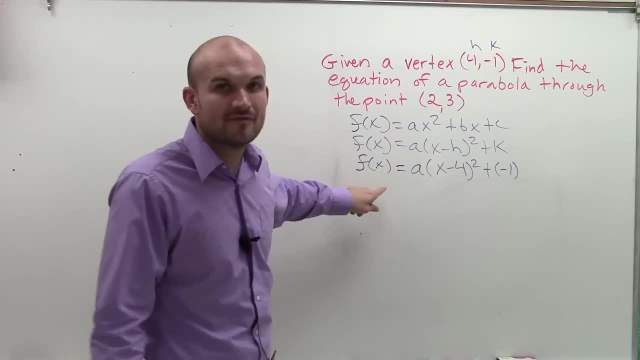 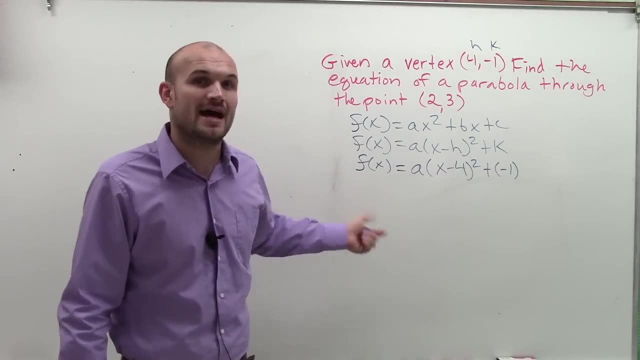 We still need to figure out what a is, and how can we represent x and f of x? Well, remember, f of x is the same thing as y, but we're talking about functions for this problem. But our f of x represents our output value, which is equivalent to y. 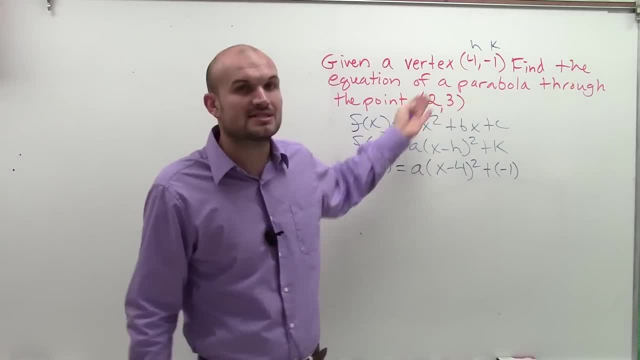 And you might want to even change it to: So f of x is the same thing as f of y, So f of x is the same thing as f of y. That might help you out understand a little bit more about it. But anyways, you can see that I have my point, which is, you know, a coordinate point. 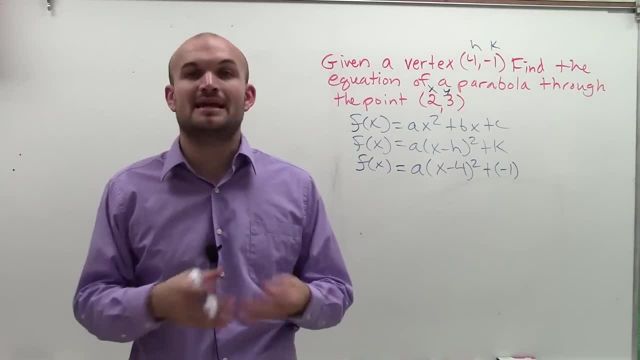 And guess what? A parabola is like a line, meaning that it's made up of infinite many points. It takes a different shape, but it's still made up of infinite many points. So I can plug in my coordinate point for x and y. 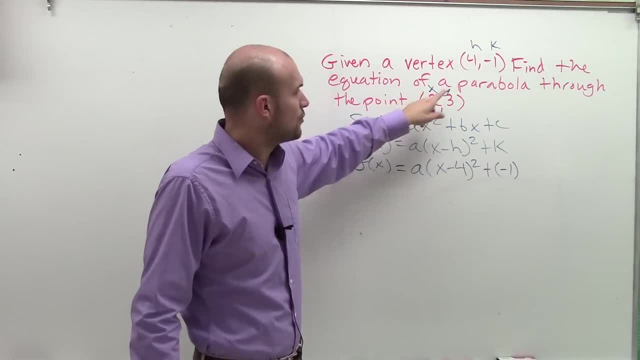 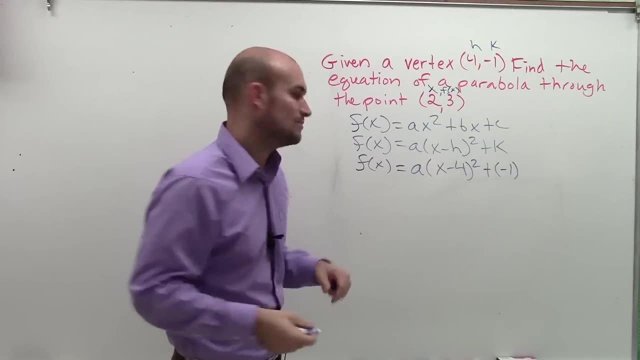 Or if, since we're dealing with a function, x and f of x. So that's exactly what you do. You plug 3 in for f of x. Still the same thing. You plug 3 in for f of x. You plug 3 in for f of x. 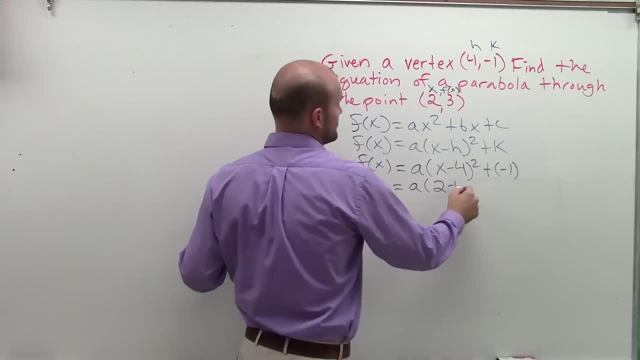 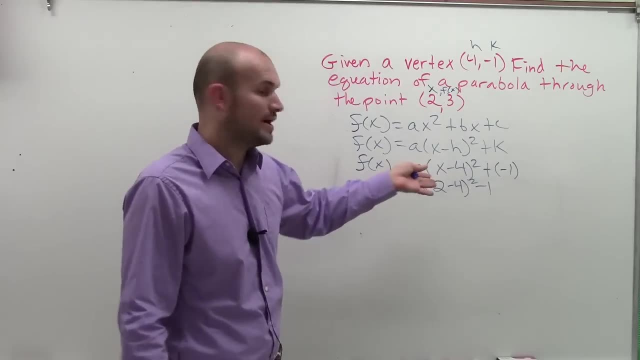 You plug 3 in for f of x. So if we want to know a, then we do 2 minus 4, squared plus a negative 1 is the same thing as minus 1.. 2 minus 4 is negative. 2 squared is going to be 4.. 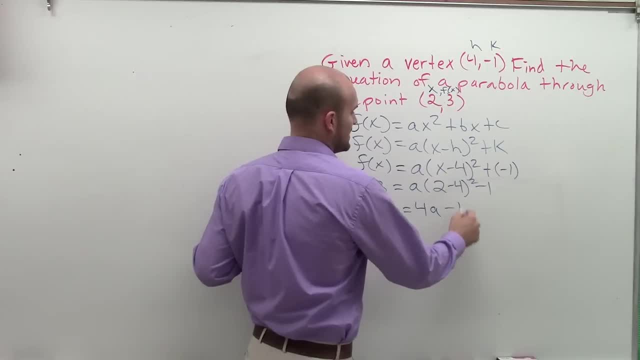 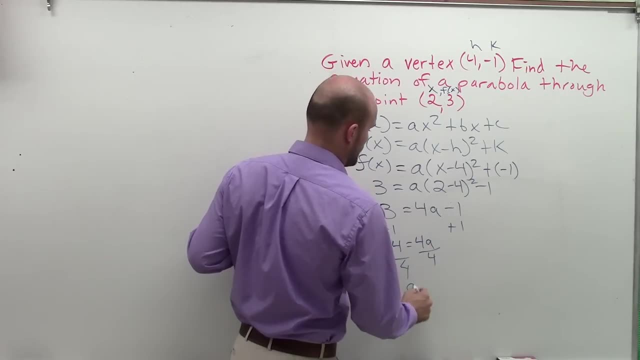 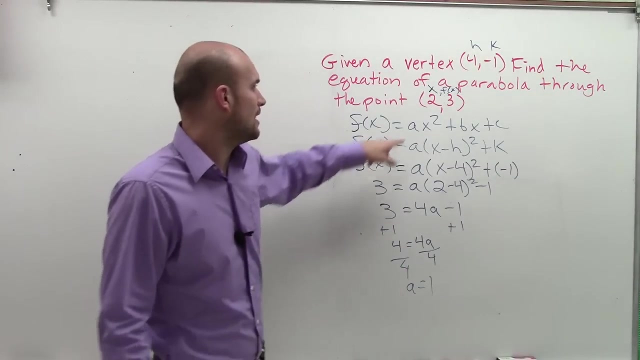 I'll rewrite the 4 in front of the a minus 1.. Add 1.. 4 equals 4a. Divide by 4.. Divide by 4. a equals 1.. So now we know the value of a. We're just going to plug it now all into my equation. 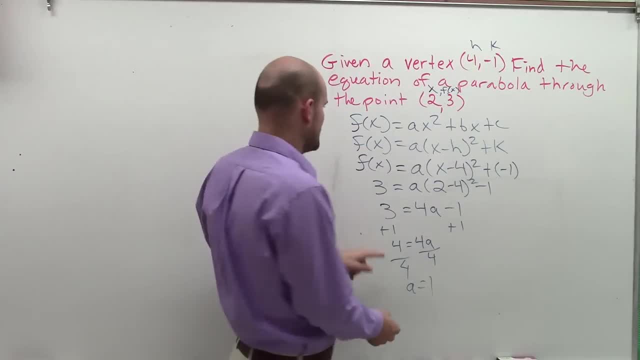 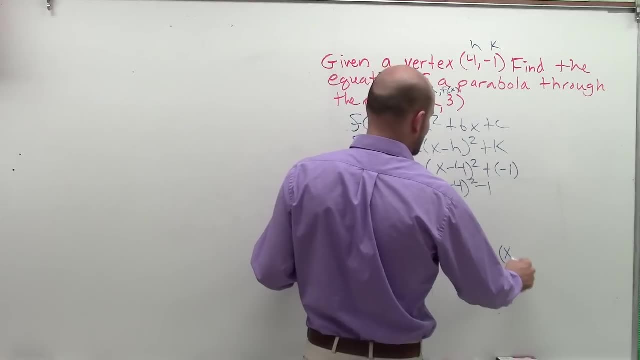 Into this equation. I'm going to write a vertex and we can leave it there. So my a is 1.. So I have f of x equals 1.. We actually don't even need to write it. Then we just have x minus 4 minus 1 squared. 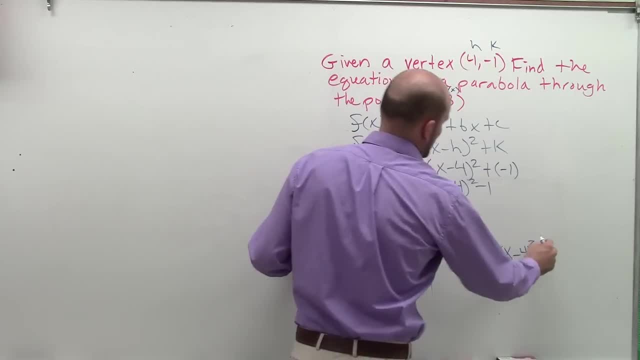 Then we just have x minus 4 minus 1 squared. Then we just have x minus 4 minus 1 squared. So there you go, ladies and gentlemen. That's how you write an equation when given a point and a vertex. That's how you write an equation when given a point and a vertex. 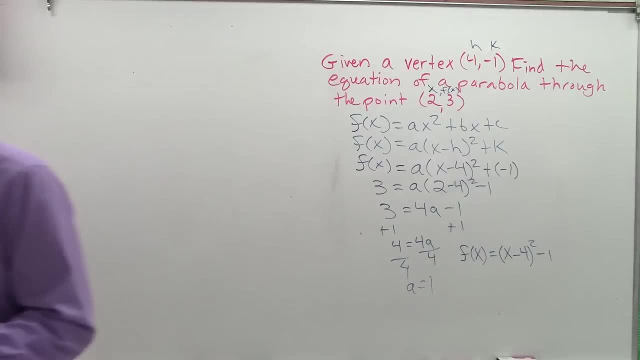 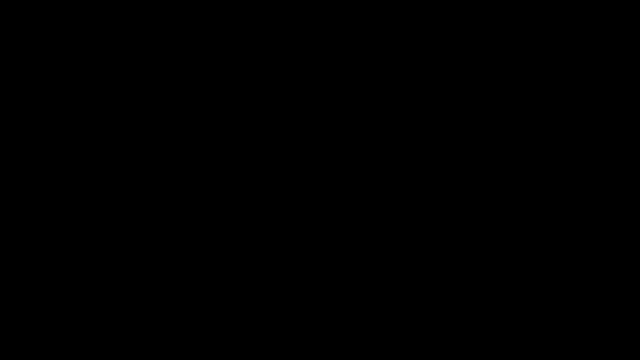 Thanks. Subtitles by the Amaraorg community. 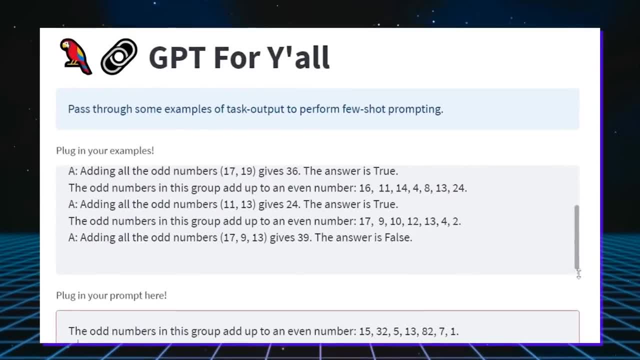 This large language model app can answer questions, complete tasks, summarize text and write and run Python code, But the real kicker, It's free. It's not using the OpenAI API, it is completely open source. In this video, we're going to be speedbuilding the app and stacking a 7 billion parameter. 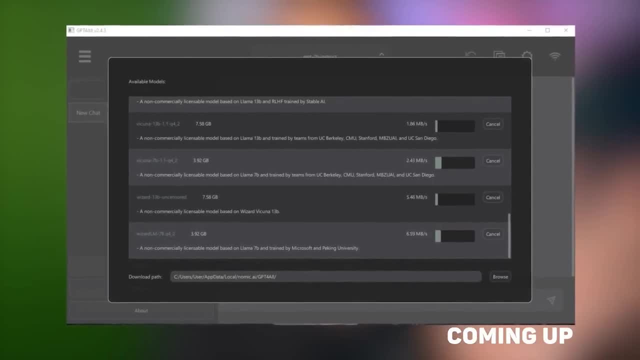 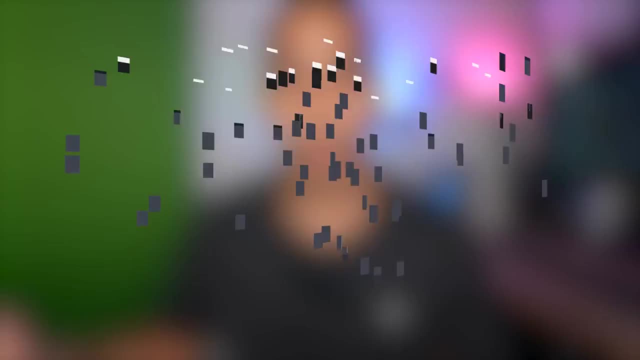 model, a 13 billion parameter model and a bunch more up against OpenAI to see if they can even get close. One of the easiest ways to get access to open source large language models is through GPT for All. Through it, you can actually use a chat-like interface whilst running the models locally. 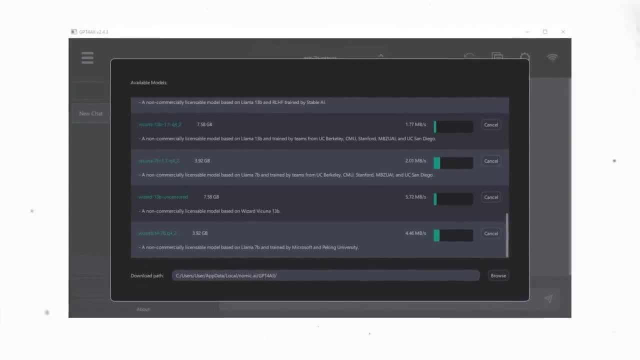 on your machine. The upside to using the GUI is that it'll actually download the model weights to your machine, which means that you can then use it. inside of Langchain. There's GUI-based installers available via the GPT for All website. 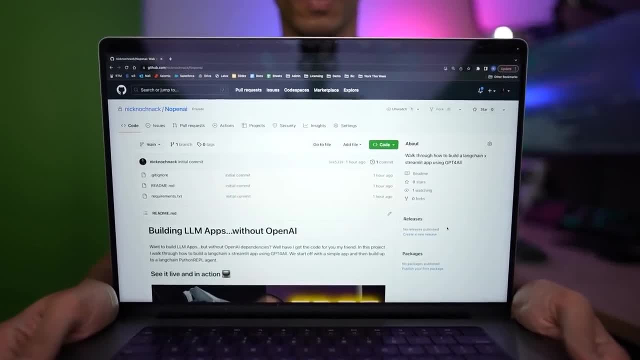 I've also included detailed steps on how to run the code if you want to get it up and running yourself. I'll get to that a little bit later. So first up, I downloaded and installed the GPT for All GUI to my Windows machine.